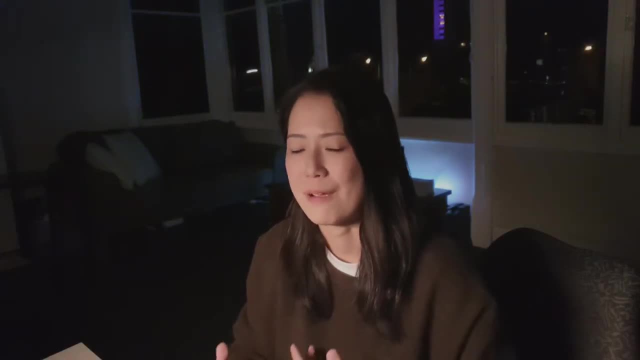 operations here, because we'll be talking about the graph search algorithms in another course that I'm planning to start. Okay so, oh, and if you like my videos, please like and subscribe. Okay so, let's get started. Let's see this tree over here. 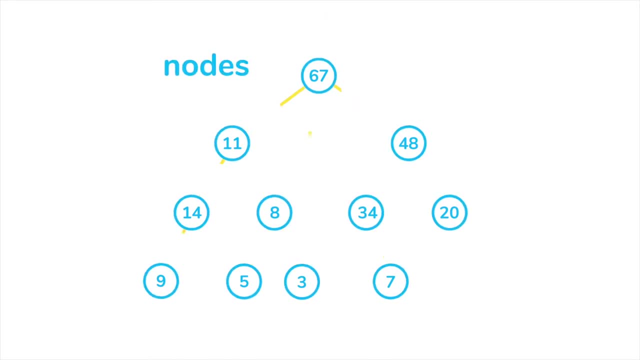 So in this tree we have nodes and we have edges, and in trees the edges point from the parent to the children. But what if we add a little bit more to this? What if these edges got a little bit crazy and started to point to other things? 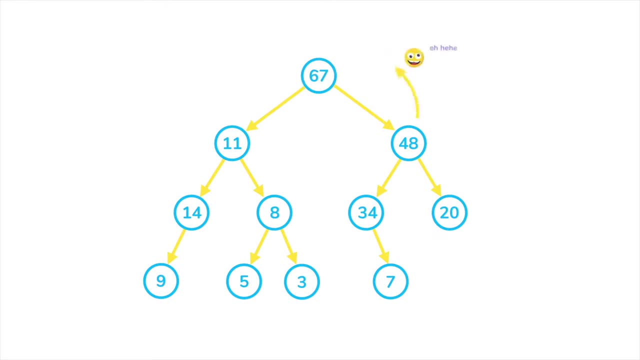 For example, a child node starts to point at its parent, And then they start to point to each other, or even point to nodes in other branches, making cycles and even pointing to itself. This doesn't look like a tree anymore, does it? We can't tell which one is the root. now, can we? 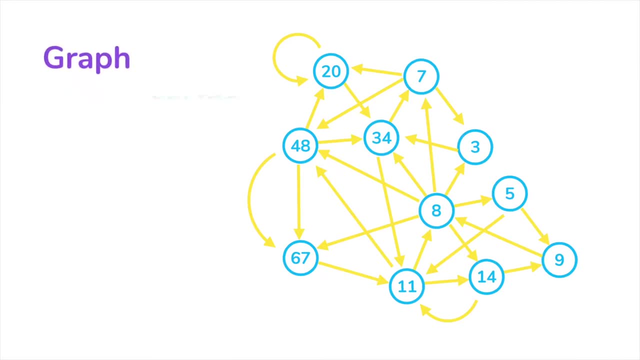 This is what we call a graph. So for graphs, we call these vertices and these are called edges. When the graph has many edges, we call it dense a dense graph. When it has relatively less edges, we say that the graph is sparse. 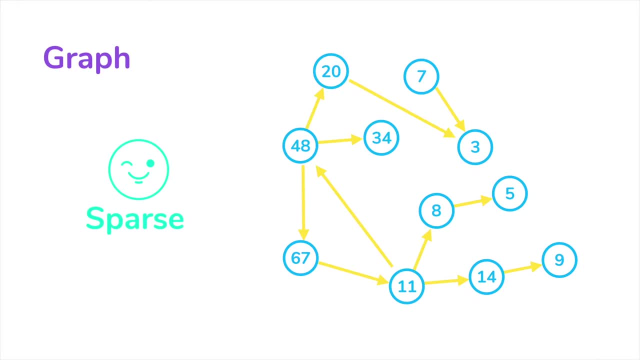 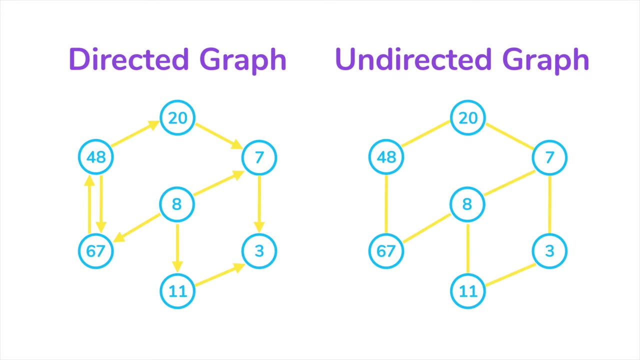 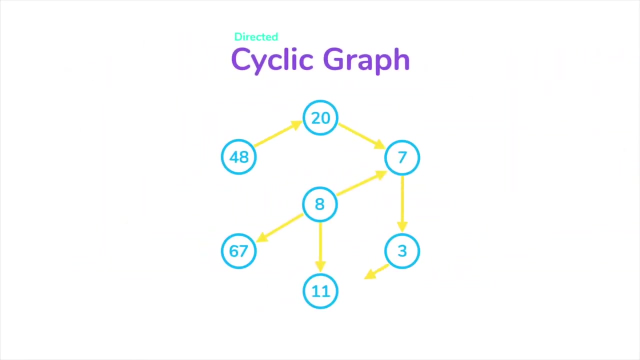 So a graph is an abstract data type, And so there are many different ways to implement it. You can make it a directed or undirected graph. An undirected graph means that every edge is bi-directional. It goes both ways. You can also allow cycles or not. 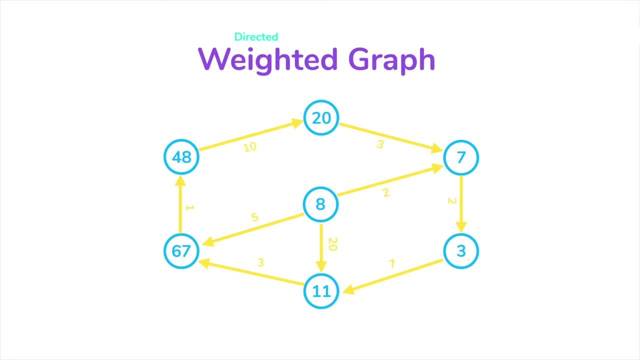 You can also put weights on the edges. For example, you can use weights to calculate the time of passing a certain path from point A to B, like finding a path in Google Maps and calculating how long it would take. You might have also noticed that the tree structure is also a type of a graph, but it has more. 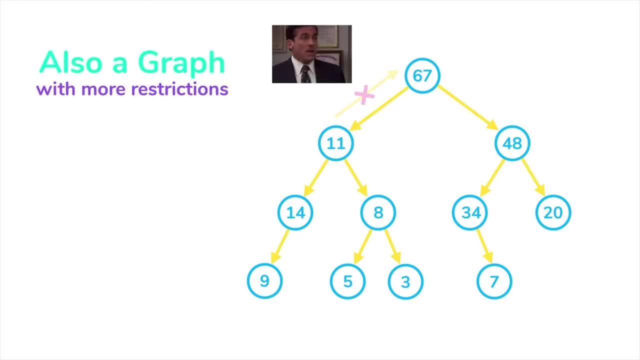 restrictions or rules like, for example, children cannot point to a parent, no cycles are allowed, or if it's a binary tree, there should be only maximum of two nodes as children, and so on. So I just want to say that there are a lot of 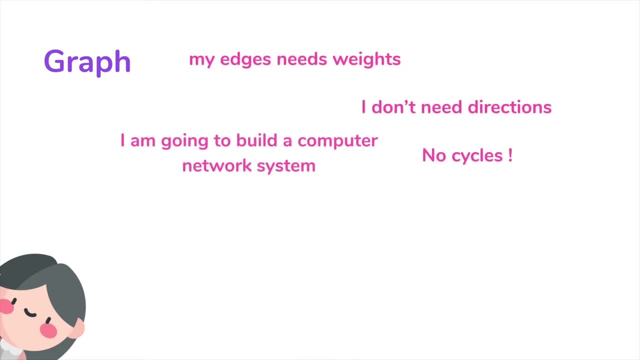 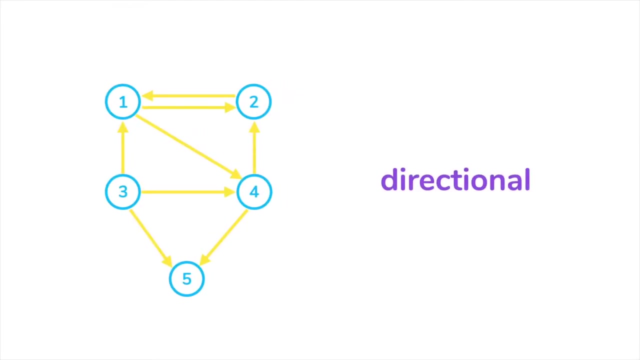 different implementations of a graph, which, when you choose, would depend on what it needs to do. Okay, so now we know what a graph looks like and we also saw different kinds of graphs. You can now tell that the graph you're looking at here is a directional graph. It allows cycles and it's unweighted. 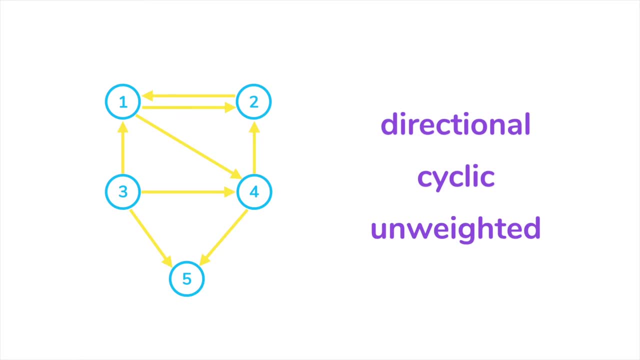 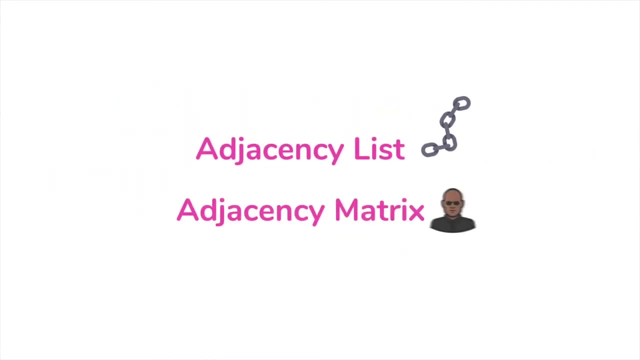 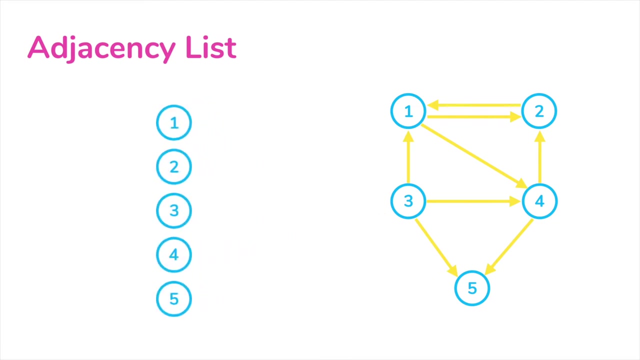 Now let's think about how we're going to express a graph in code. There are two common ways to represent a graph. One would be the adjacency list and the other is going to be the adjacency matrix. So for an adjacency list, the graph is expressed as a list of vertices, and 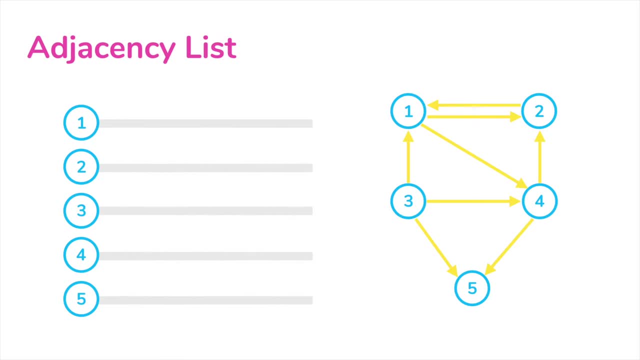 each vertex will have a list holding the neighboring vertices, So it's going to look like a list of lists. These lists can be a link list or arrays, dynamic arrays, anything that can implement a list. We will call the integer values of the vertices keys, and if they're going to represent a set of information, 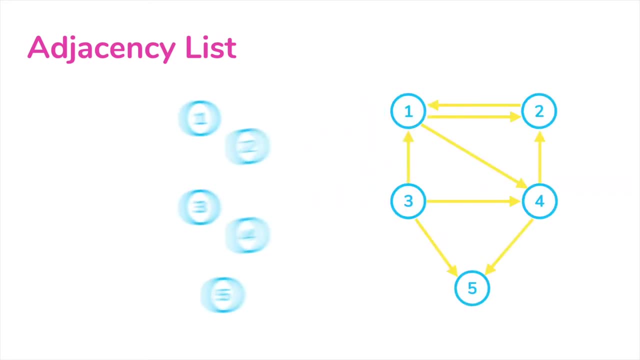 they should be kept. that way be unique. Okay, so let's start filling in the adjacency list. If you see the graph a, 1 is pointing to two vertices, 2 and 4, so these two should be in the adjacency list for 1.. And same goes for vertex 2, it's pointing to 1, so there should be. 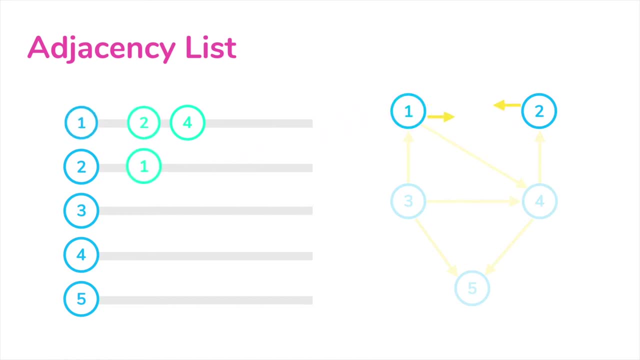 vertex 1 in the adjacency list of vertex 2.. Do you see how 1 and 2 are pointing to each other? So if this was an undirected graph instead of a directed graph, all the vertices should be looking like this: if 1 has 2, then 2 should have 1. 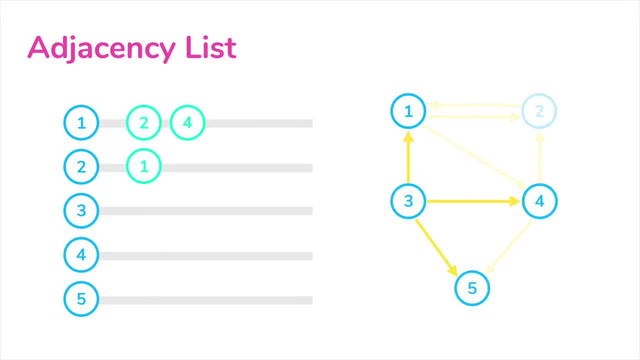 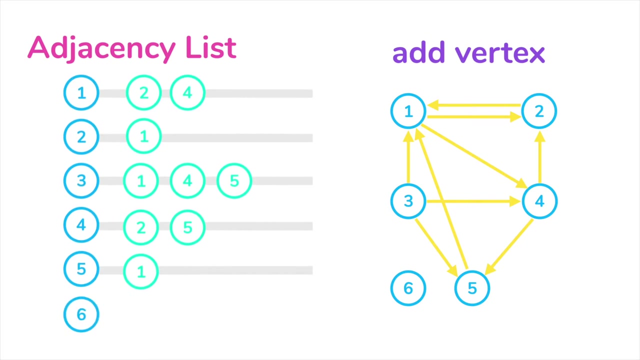 if 1 has 4, then 4 should have 1.. When we want to add a new edge to the graph, we can just add a new element to the adjacent list, and when we want to add a new vertex, we just need to add a new vertex to the graph list. Okay, so that is. 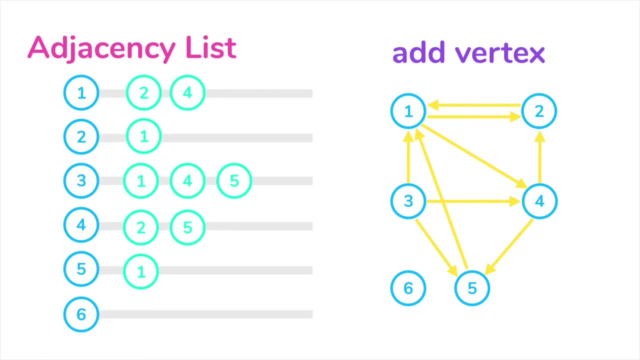 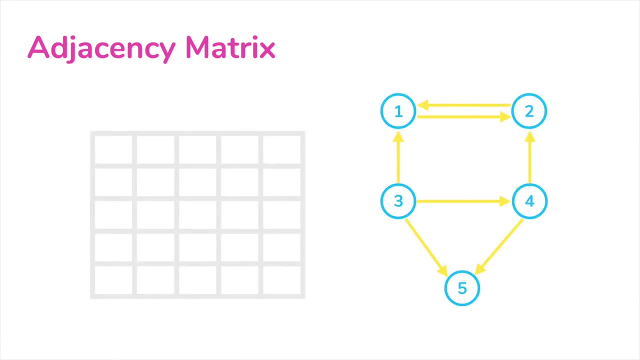 how you can represent a graph with the adjacency list. Now, let's look into the adjacency list. Let's look into the adjacency list now. Okay, so let's start. matrix: We can also express a graph structure with a two-dimensional array. We'll put the vertices of the graph as columns and rows and they're going to 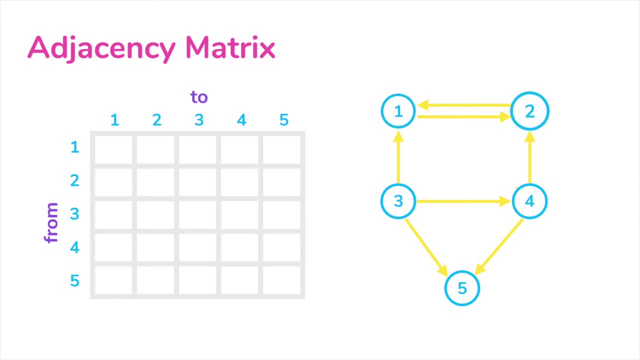 represent the from and to vertex. For example, if we have five vertices in the graph, we would need a matrix of 5 by 5. And here there is an edge connecting from vertex 1 to 2, so that entry from 1 to 2 would be 1.. And same goes for every. 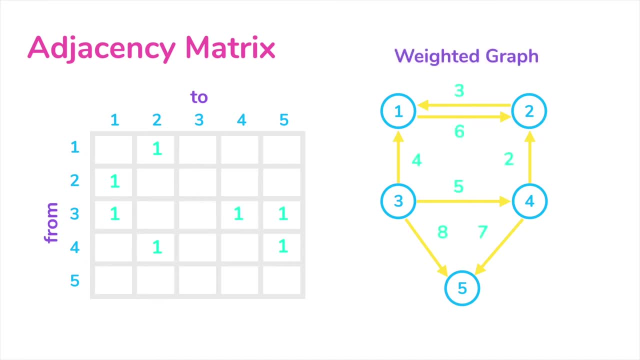 other edge in this graph And if this was a weighted graph, the entries would hold the weight instead of just holding 1.. If we have an undirected graph, the matrix would be symmetrical, because undirected graph means that all the edges are. 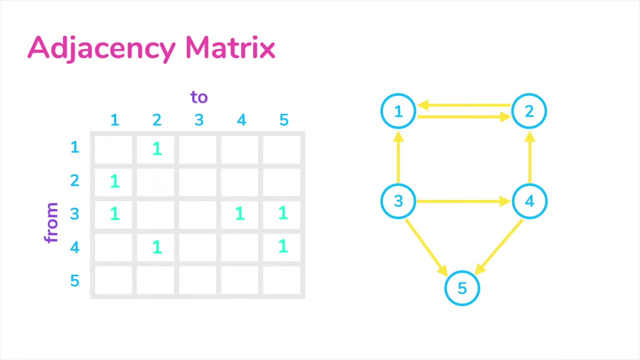 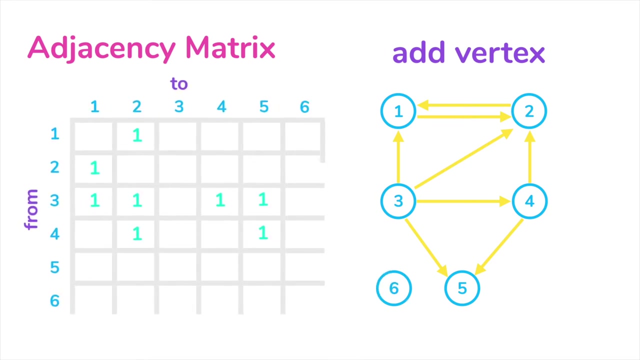 actually bidirectional, Okay, so let's go back to the directed unweighted graph and see how we can add things to it. If you want to add an edge, you just need to fill in the from and to vertices, And if you want to add a vertex, you'll have to add a row and a column. but 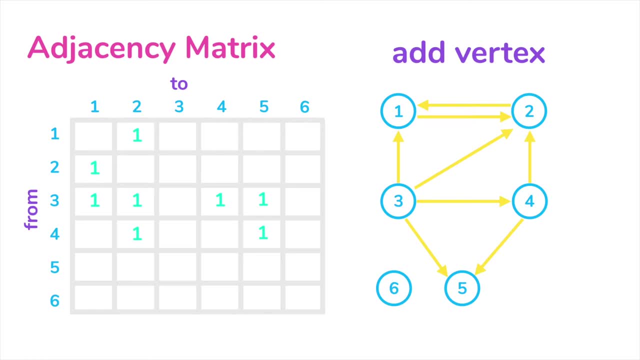 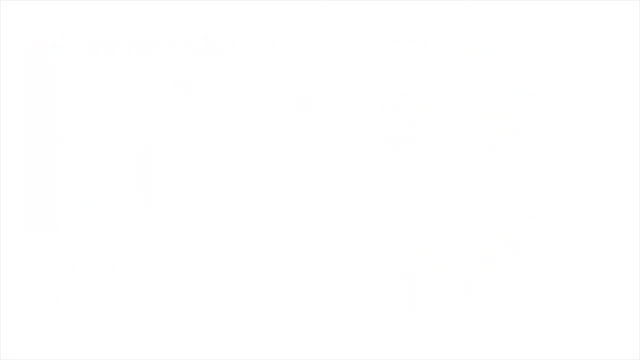 actually, you just can't add dimensions to a matrix. You'll actually have to make another one and then copy all the elements inside it, And we'll talk about that a bit more later on. Now let's compare the two, adjacency list and adjacency matrix. First of all, which? 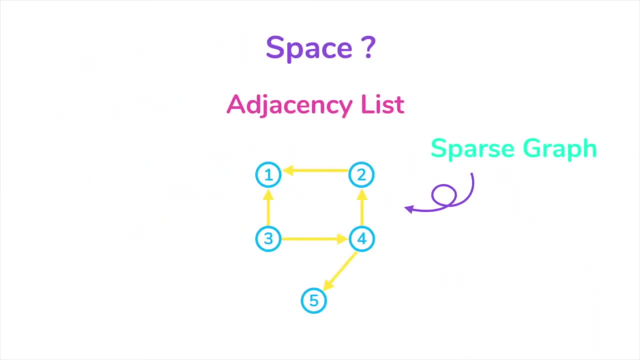 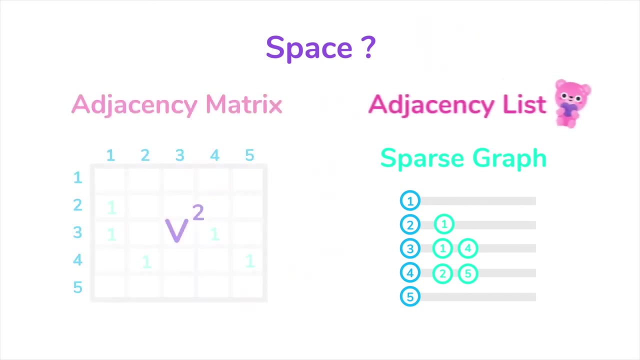 one do you think would take less space? If the graph is sparse, using the adjacency list can let us save space, but for an adjacency matrix you will always need a space for v squared where v is the number of vertices. no matter how sparse the graph is, you'll need that much space. what? 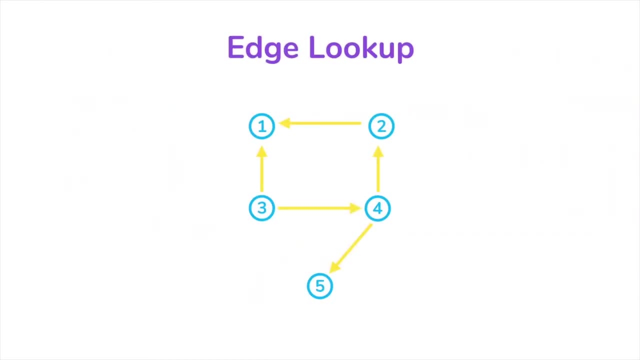 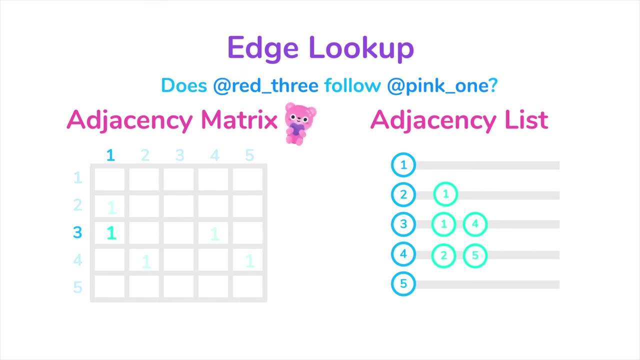 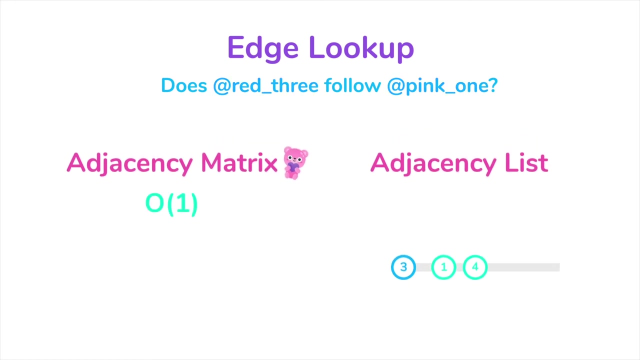 about looking up an edge, like checking whether two vertices are connected or not, or checking whether who follows who. in that case the adjacency matrix is much faster because we just need to do an array lookup, which would just take constant time. but if you try to do that in an adjacency list, we need to. 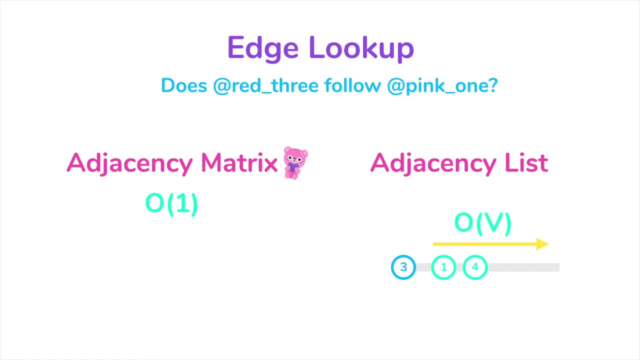 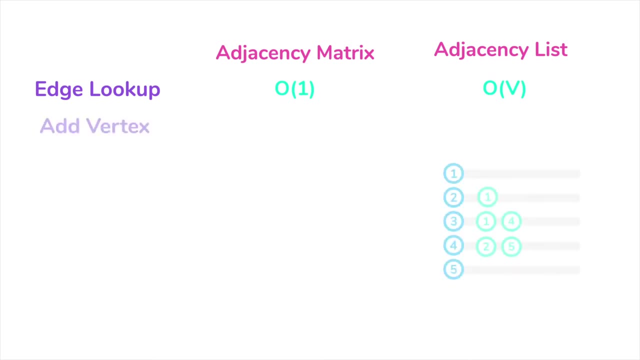 traverse the list of adjacent vertices, which, in the worst case, we would need v steps if the number of vertices is v. let's think of some other operations. adding a vertex could be easily done in an adjacency list, because we just need to add an element to the list, but for the adjacency, 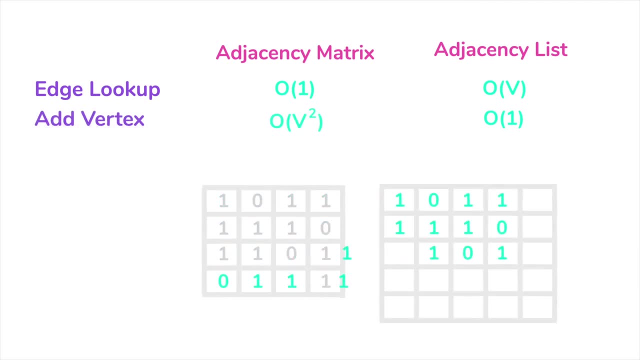 matrix. we need to copy the whole array of vertices to the adjacency matrix and we need to copy the whole array of vertices to the adjacency matrix. and we need to copy the whole array of vertices to the matrix which would be o of v squared. that goes the same for removing the vertex too. we need to.